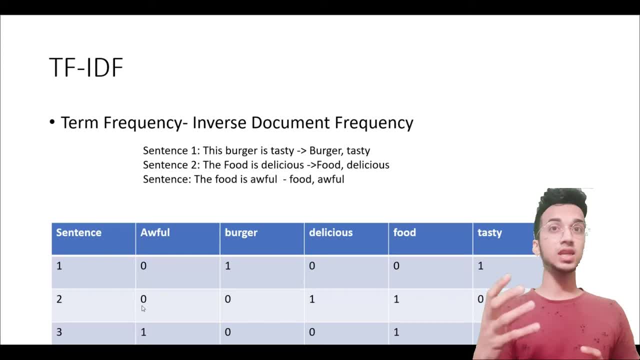 a continuation, So let's talk about this method first. So this is basically a method for converting words into vectors. right? We talked about word vectorization in previous videos. Whenever you want to train a natural language processing model, you need to convert those words into. 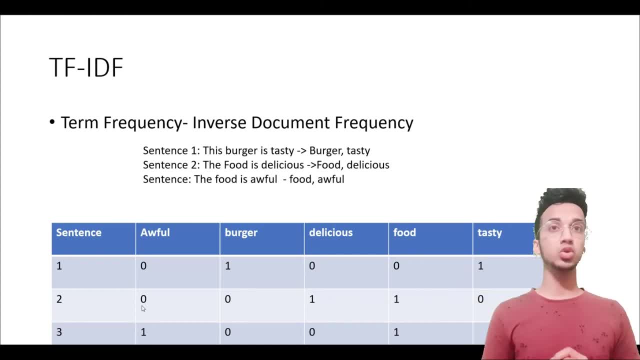 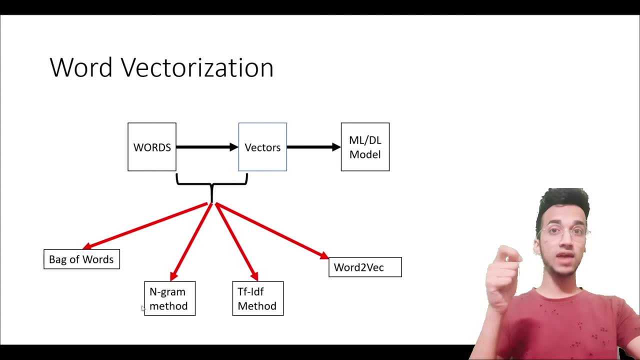 numbers, right? So TF IDF is just one method to do that. In my previous videos, we've discussed that. to convert words into vectors, there are four methods, right? So I've discussed bag of words before. In this video I'm going to discuss TF IDF, So let's look at what it. 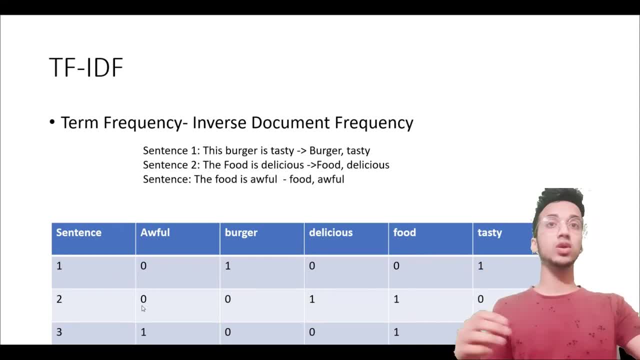 exactly does So. in the bag of words approach we saw that whenever you have a sentence say this burger is tasty, the food is delicious, the food is awful, First step normally is to remove the stop words, right Words which do not have any result on the meaning, like 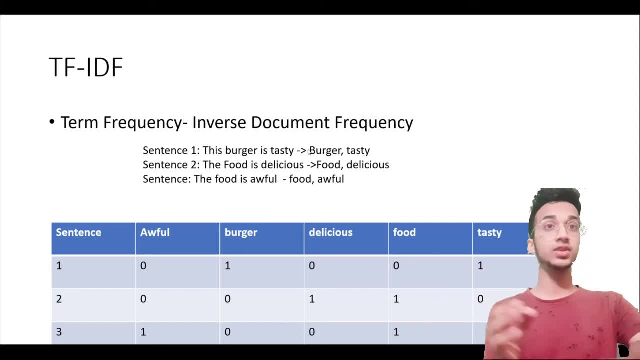 this, This is the. so you get finally these words: burger, tasty food, delicious food, awful, And these are the words that you will be supplying to the model. So in bag of words approach, we saw that to represent any sentence, we simply update the corresponding frequency. 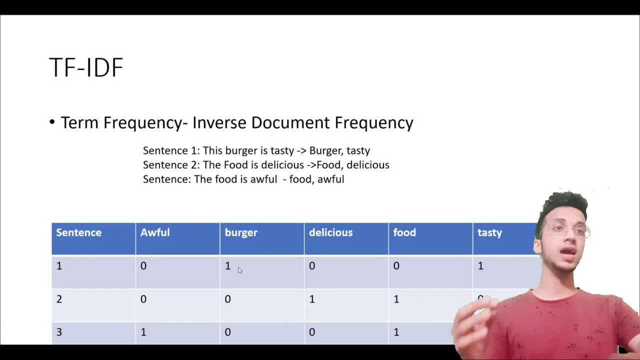 of the word. like in sentence word burger is present once and tasty is present once. I rest. all the words are not present, So they're denoted by zero, Similarly, for each sentence you represent this way. So problem was that you're not able to give. 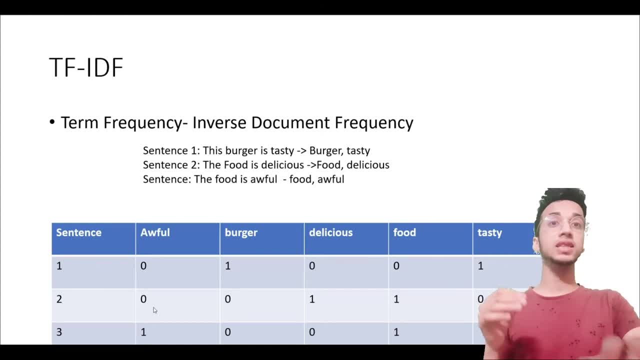 weightage to important terms, right. For example, in this particular scenario, tasty is very important, right, or delicious is very important, right. They are conveying the sentiment. So in this scenario, tasty and burger have the same importance. Also, if words like the 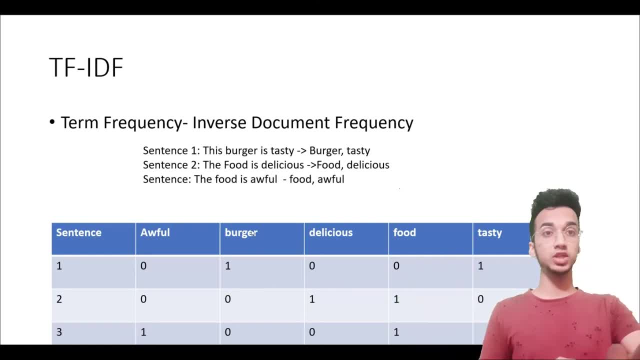 and is were not removed, they would also have a very high weightage because their frequency is a lot in the document. So basically, term frequency is what it's- number of times a word is occurring in a particular sentence. right Now, when the word is occurring a lot, it might get very high importance To prevent that. 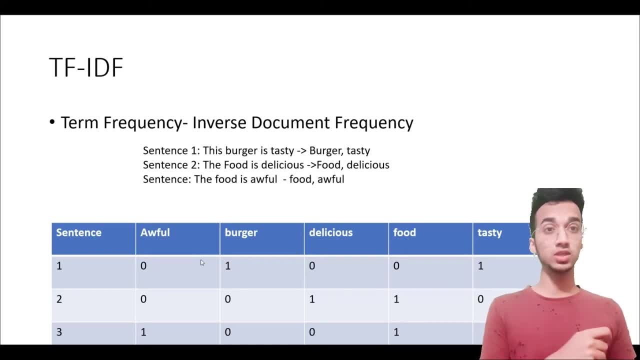 from happening. we introduce something called as the inverse document- frequency. And now let's look at the formal definition, And I'm going to give you an example, And it's going to become very clear after that. So, in this case, how does this method work? you first. 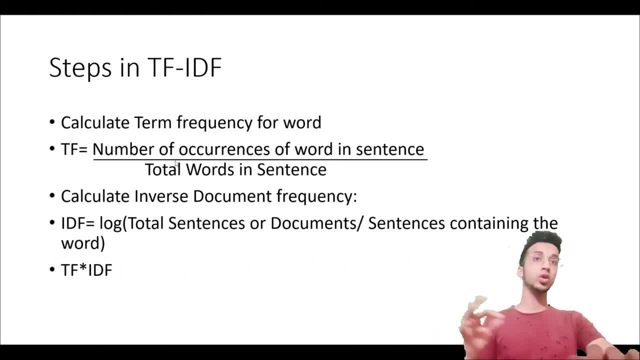 calculate the term frequency for a word, which is given by the number of occurrences of a word in a sentence divided by the total number of words in the sentence. That is the method for finding the frequency. Once you find the frequency, you also have to find something called as the inverse document. 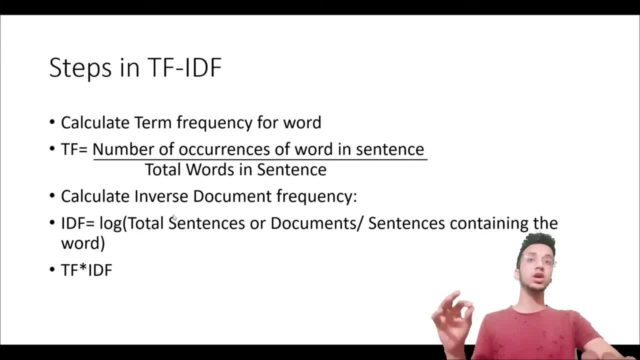 frequency right. It's given by this formula: log of total number of sentences, or it's also called as documents, So total number of sentences divided by sentences containing the word right. Why do we do this? When I show you the example, this will become more. 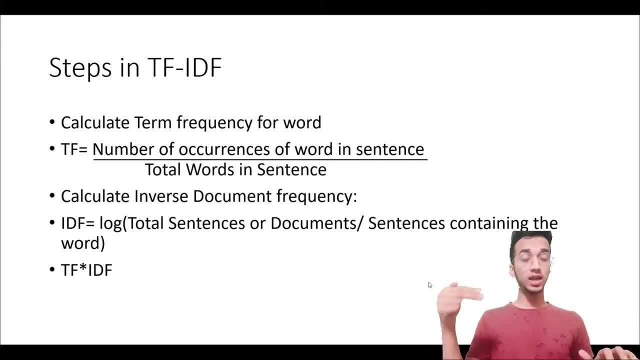 clear Basic goal is that when a word is occurring again and again, it will, it will get very high weightage because it has high frequency. We multiply it by the IDF. So finally, take the TF and IDF for a particular word and use: 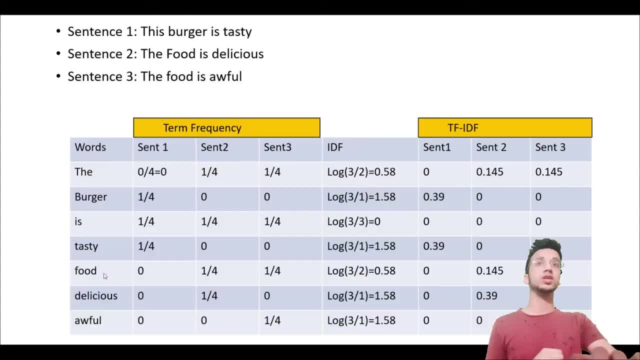 that for representation. So let me show you the actual working of this right. So let's go back to those three sentences: This burger is tasty, The food is delicious, The food is awful. In this case, I'm not going to remove these stop words, because I want to illustrate. 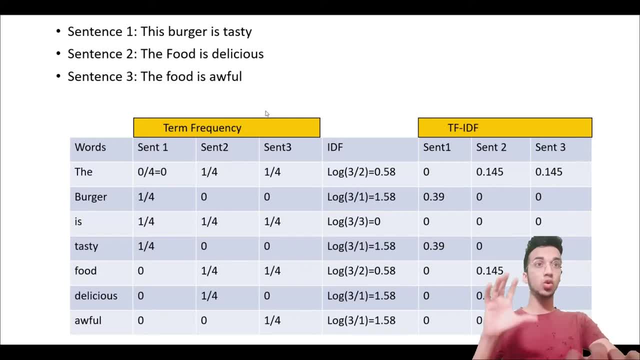 how TF IDF exactly works, right? So what is the process? for each word, You have to calculate the term frequency. So in my left-hand column I've listed all the words, right? So what is the process? for each word, You have to calculate the term frequency. So in my left-hand 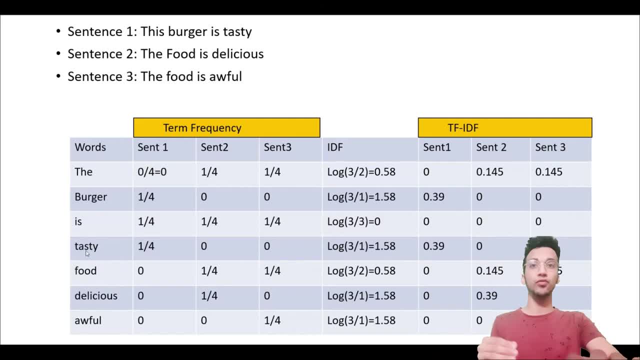 column. I've listed all the words, right, So what is the process for each word? You have listed all the words right, So what is the process for each word? You have to calculate the term frequency, right? So in this case, you have to calculate the term frequency for. 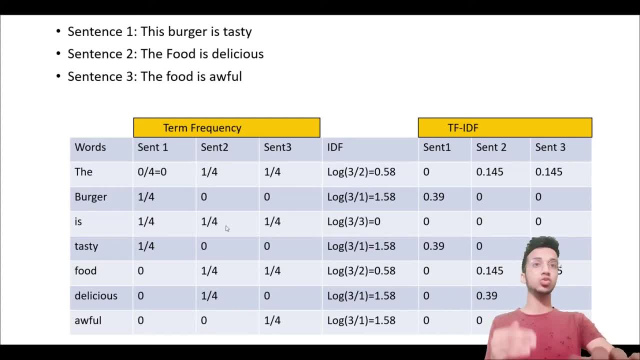 each sentence as well. So if you look at the first example, sentence one, and the word there, since there is not present, it's given a zero divided by four, which is equal to zero. Similarly, in sentence two, there were, the is present once out of the total four words. 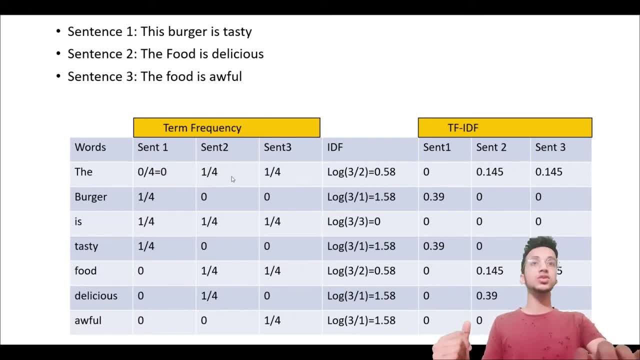 so it's frequency as 1 by 4.. Similarly, in sentence 3 also it's present 1, so it gets 1 by 4.. Similarly for all words we have done, this Burger is present in sentence 1 and it's one word out of the. 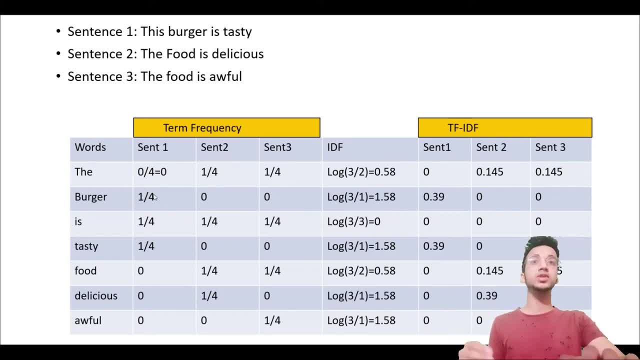 four words, so it gets frequency of 1 by 4.. It's absent in the rest two sentences, so we write 0 and 0. In this method you calculate term frequency for each word in different sentences. Step number 2 is to calculate the IDF inverse document frequency Now inverse. 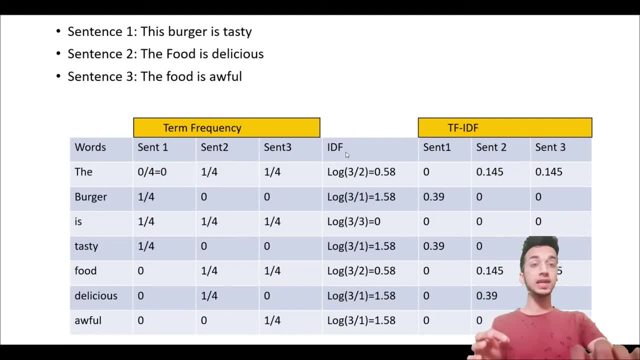 document. frequency is going to be same for all sentences for a particular word, So the formula becomes log of. in numerator you have the total number of sentences, which is 3 in this case. and for the word the, the is present in sentence number 2 and sentence number 3. 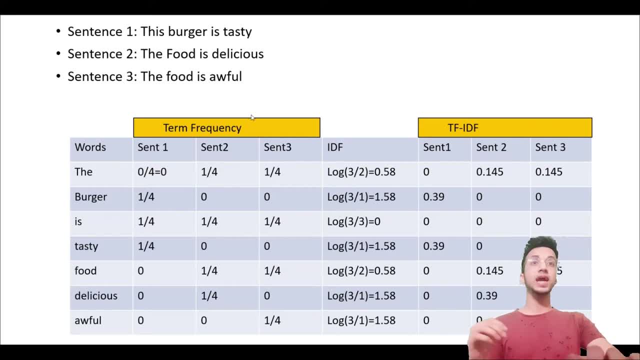 which means it's present in two sentences. So we write as log 3 by 2 and this is to the base of 2, so you get a value of 0.58.. Similarly for burger it's present. total number of sentences is 3.. 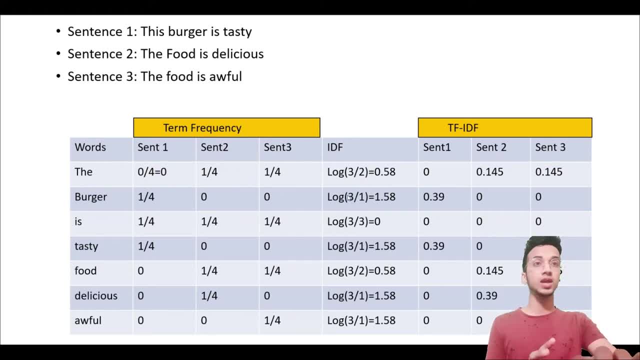 And it's present in one sentence. so we write 3 by 1 and the value equals to 1.58.. Similarly for is, we get log 3 by 3 because total number of sentences is 3 and it's present in all the three sentences. So after you have calculated TF and IDF, you have to multiply that. and for: 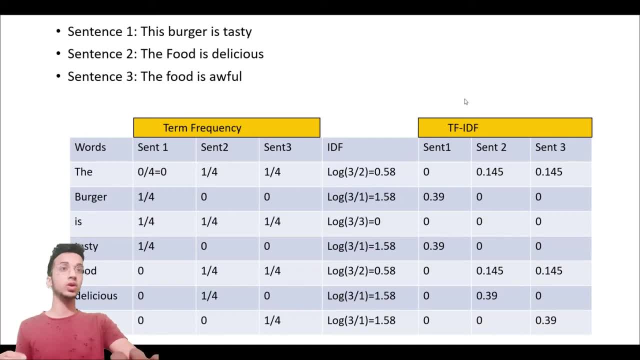 each sentence you will get a different vector right. So let's say, for sentence 1, how do we finally get the vector representation of sentence 1.. So, sentence 1, you take the first word, the Frequency, which is 0, you multiply it by the IDF, so you get 0.. The next word in this row. 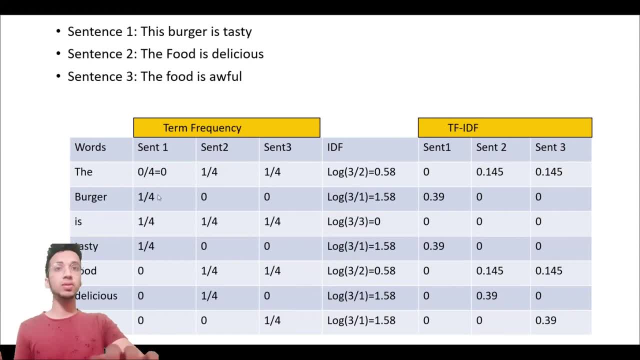 is burger, right? So in sentence 1 this frequency is 1 by 4 and IDF is 1.58.. So you multiply these two and you get 0.39.. Similarly for, is you multiply 1 by 4 by 0, you get 0.. For 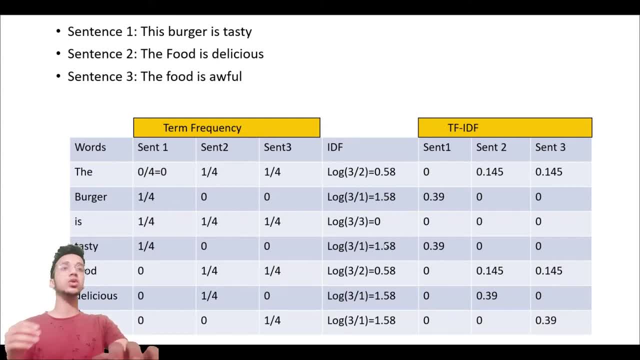 tasty. you multiply 1 by 4, by 1.58 and you get 0.39.. And you do this way for all the sentences. So on the right hand side, TF, IDF, these three, these three columns is the number of sentences, is what you're going to supply to your machine learning model. right Sentence? 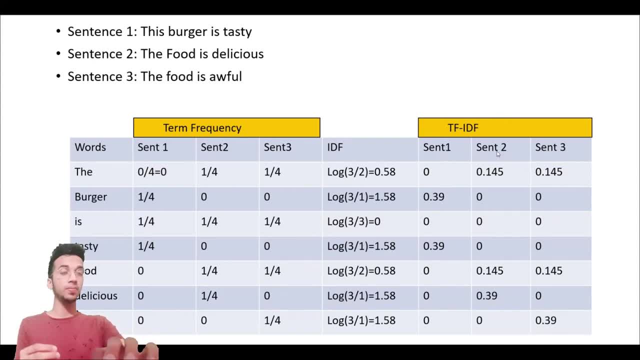 1 is represented this way. Sentence 2 is represented this way. right, And what was the benefit? So let's see: the word is right. The word is was a very useless word, right, It should not have any weightage at all, right? So the word is has a weightage of 0 in all three sentences. 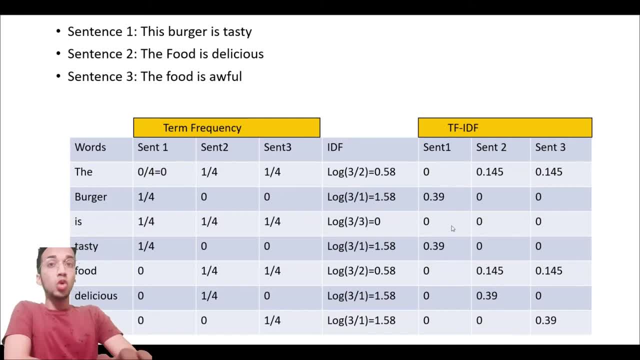 right, Because the IDF for that was 0.. So what? whatever was more important in your document, they are going to be given as High weightage, and words which are not important they will be given low weightage. So let's take sentence 2 right? Sentence 2 was: the food is delicious. So in this delicious was, 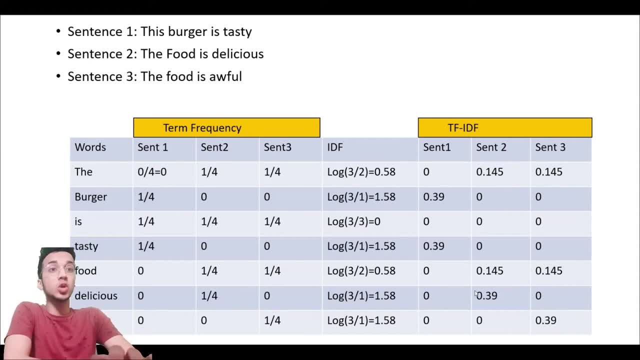 very important in conveying the sentiment. So it has been given a 0.39 score and the rest two words, food and the- are given comparatively less weightage: 0.145 and 0.145.. So basic concept is if a word is occurring very rarely, it would normally have gotten a very low weightage. 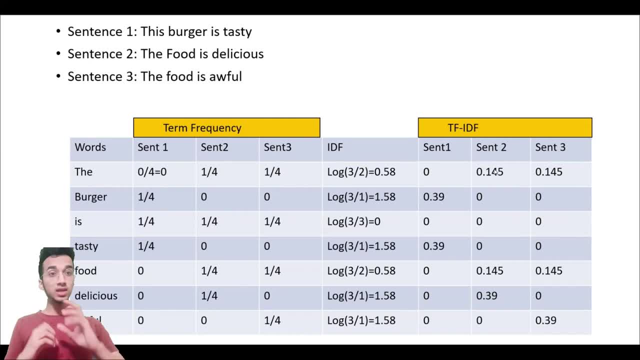 Because if it has appeared between 10 or 12 sentences, then IDF is introduced in that example where any word would be appeared in this example And presencegood activity would be a very low frequency and that low yet is consequence to negate that effect. IDF is. 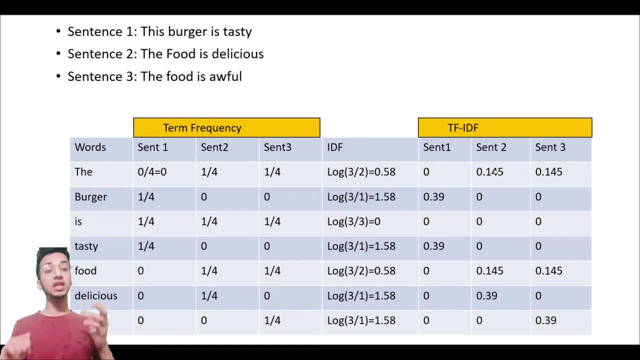 introduced. So basically, whatever word is occurring, lower, it will increase its weightage. whatever would is occurring, a lot IDF is gonna decrease that weightage. So that was it for the explanation. Now I'll show you how to implement this in python as well. So 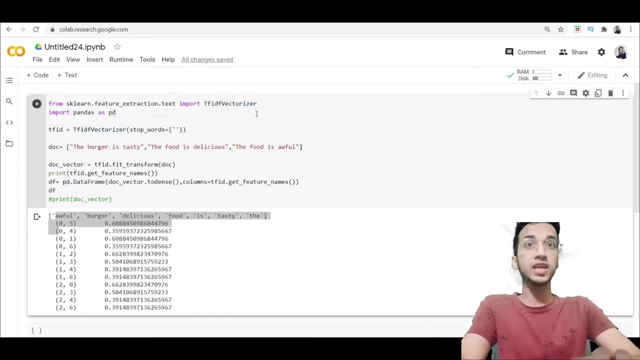 there is the python core right. first step is import the function tf Idf vectorizer from sklearnfeature underscore extraction dot text. They are also importing the pandas Library. A question must be asked in this particular case: what is the main low frequency? now I will show. 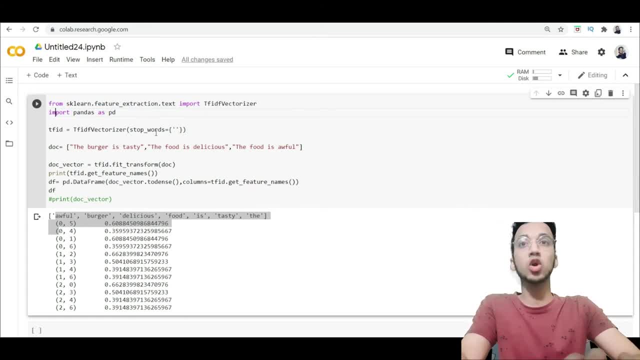 right. first step is to create an object. right, we create an object over here, store it by the name of tfid. you can give a lot of parameters over here, like stop words. if there's any particular word that you want to remove, you can add it over here and you can have a look at the rest. 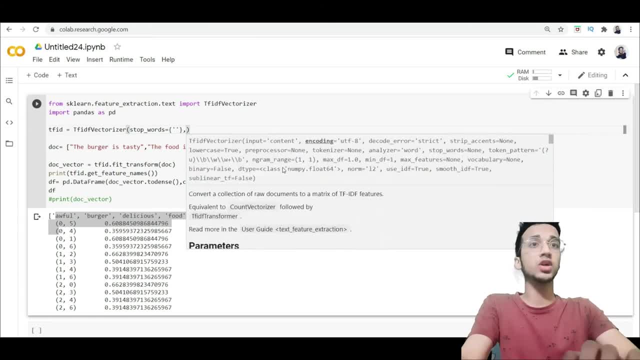 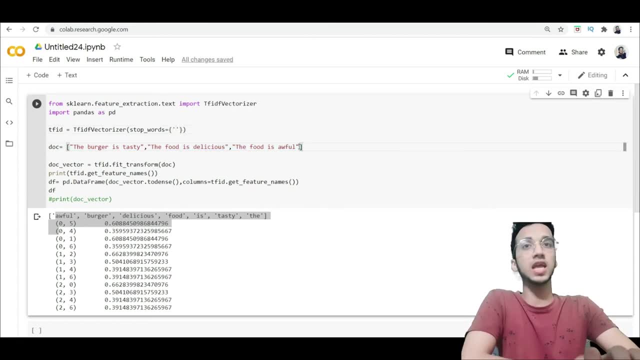 of the parameters as well. right, there's many features in this function that you can have, but for now we're not using them, right? so let's say you have a document like this. you have three different sentences, like i showed in the presentation. the burger is tasty, the 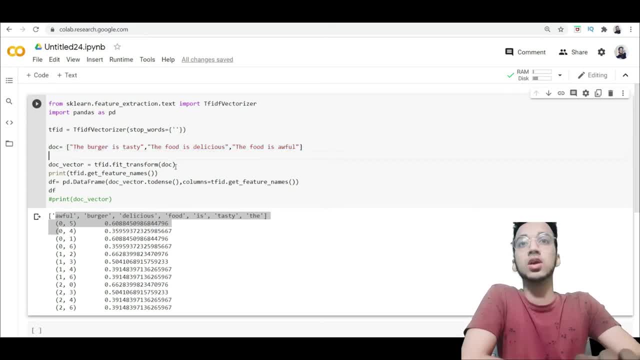 food is delicious, the food is awful, right? so we first call the function fit underscore transform and we supply the document to it and i am storing it as doc underscore vector. and when you do tfid, dot, get feature names, you can see all the different words, all the 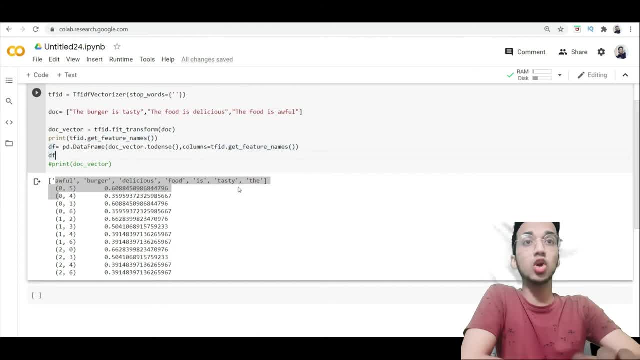 features that it's considering and these are the columns that it's gonna consider. awful burger, delicious food is tasty, the now. if you want to see the final matrix representation first, you have to convert that into a data frame. right, why? if you simply want to see what fit, underscore, transform. 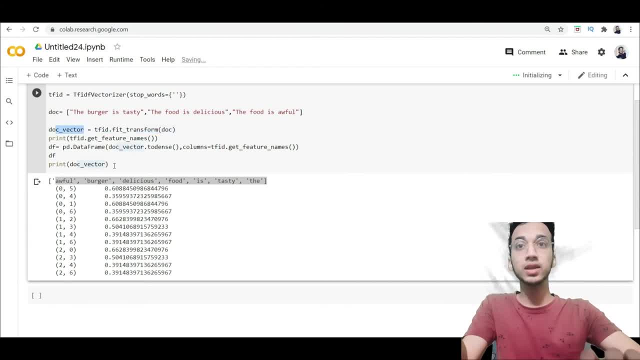 does right, which is stored in dot vector. if you simply print it you will find this right. so you will see this does not make much sense. so basically, over here we have the tf idf value on the left hand side. these are the coordinates in the matrix. so 0 comma 5 basically means uh, 0th row and 5th. 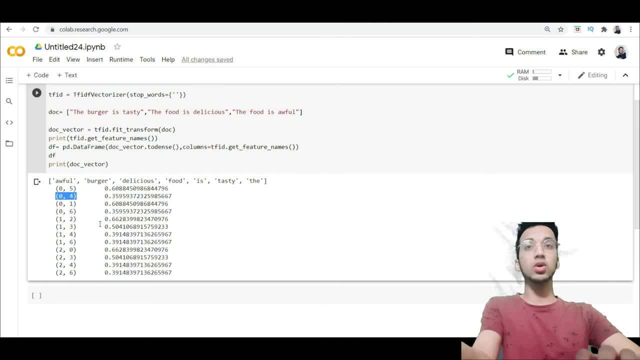 column right and 0th row and 4th column. but it's difficult to understand this way. so we call the too dense function over here, which converts that into a matrix representation, and we assign the column names as all these words and we convert that into a pandas data frame. so now, when you 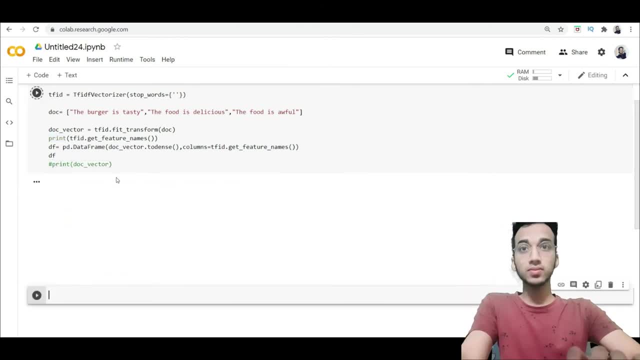 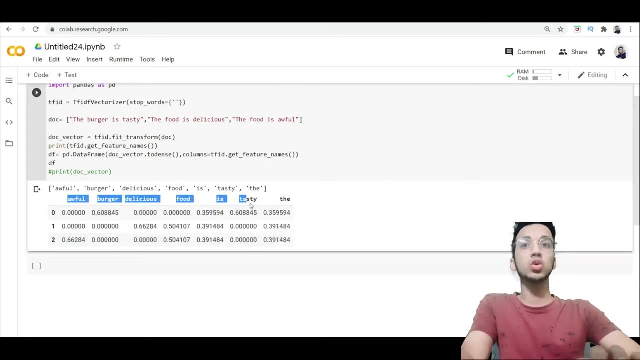 print that data frame and you run this code. this is what you'll see, all right. so, as you can see, for each word you have its particular tf idf value for different sentences. so 0 is basically the first sentence, first is the second sentence, 2 is the third sentence. right, and these values are slightly different from what we 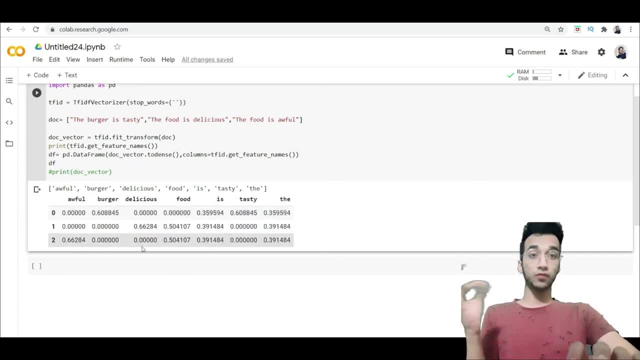 got in the presentation because sklearn uses a slight variant of the formula right. like for idf, we use log of number of documents divided by the number of documents containing the word right. so it uses slightly different variant. it uses log of n plus 1 in the denominator. it also adds a plus 1. 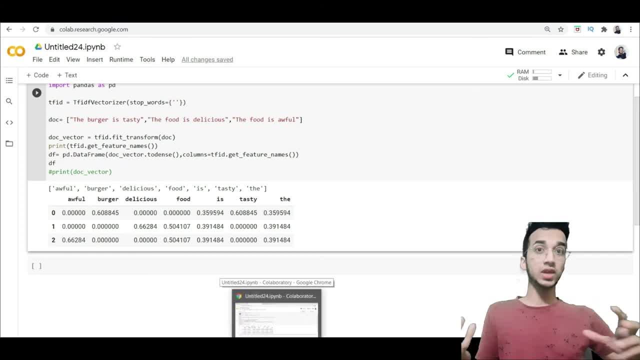 it doesn't matter. every library could use a slightly different variant of the formula. right, so we can take the burgers, but you can, or you can, change the size. consultants allowed you to do so, right? so if you look at sentence number zero, the burger is tasty, you'll see. burger has a high 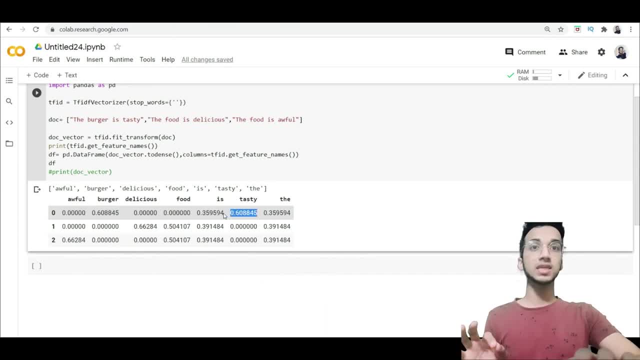 weightage. tasty has a high weightage and the words is and the word the have a low weightage. that was our goal right to assign weightage more cleverly. sentence number one, you can see delicious has the highest weightage because it's determining the sentiment right and food has a 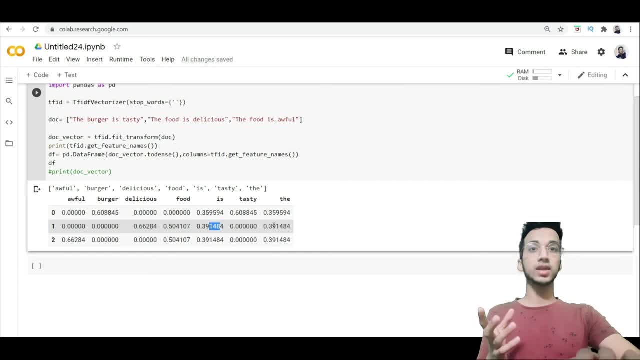 comparatively lower weightage, and is and D have the lowest weight. Similarly for sentence 3 as well, awful will have the highest weightage. So that is all about TF-IDF. it's just a more clever way of assigning weights to more important features, which we weren't able to do in the bag of words approach.